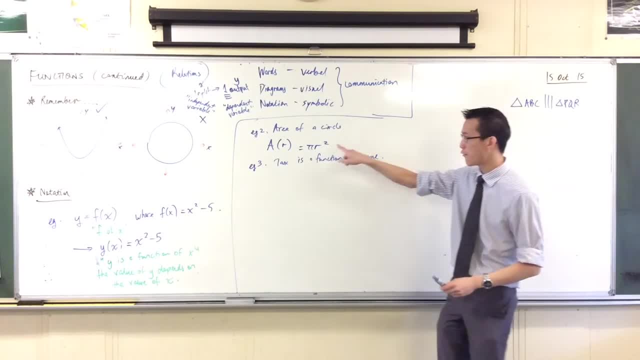 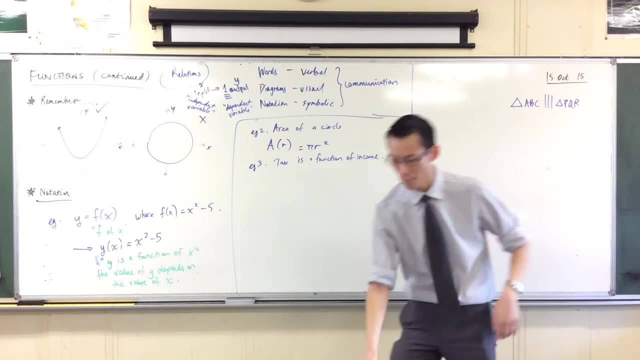 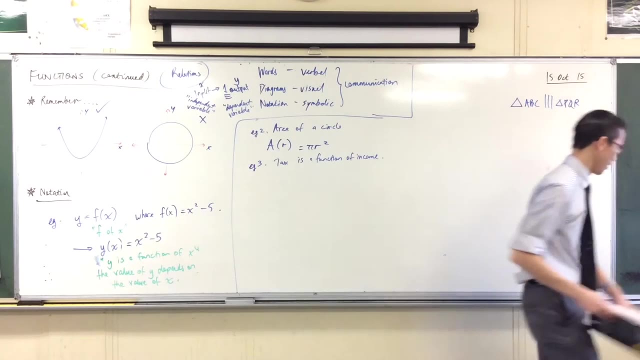 Now, the reason why I put this one out is because you know, functions can be very simple, like just a few characters, right, But sometimes functions are wildly complicated. In fact, do I have? I have it here, right, Let's see. Da, da, da, da, da, da. Yeah, perfect, Okay, Twenty-nine. 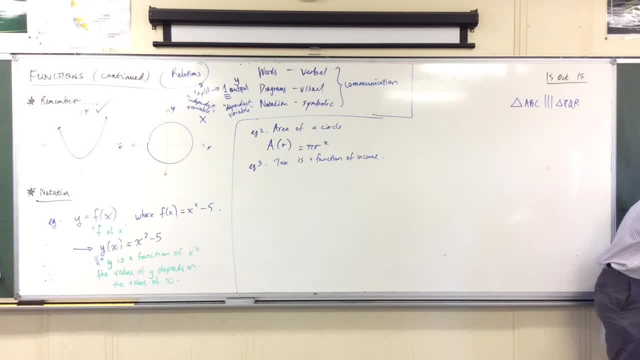 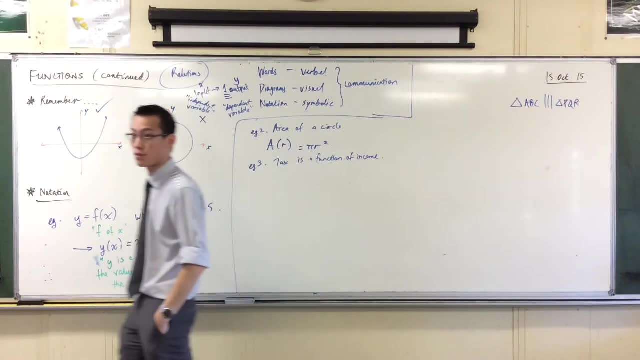 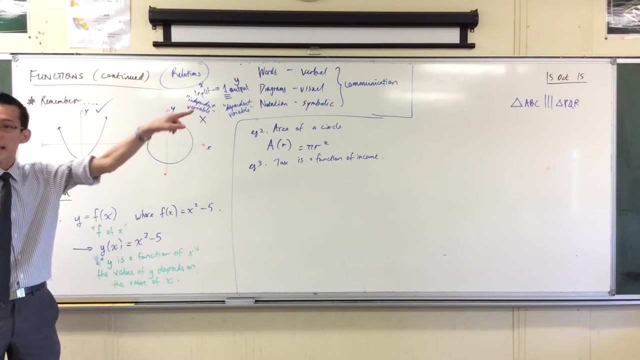 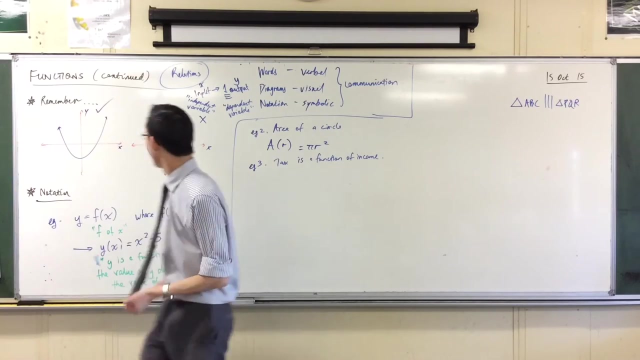 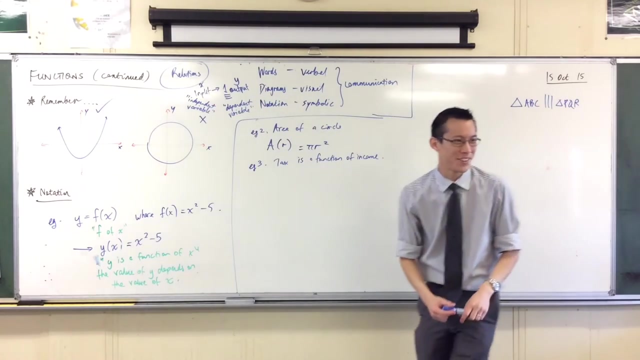 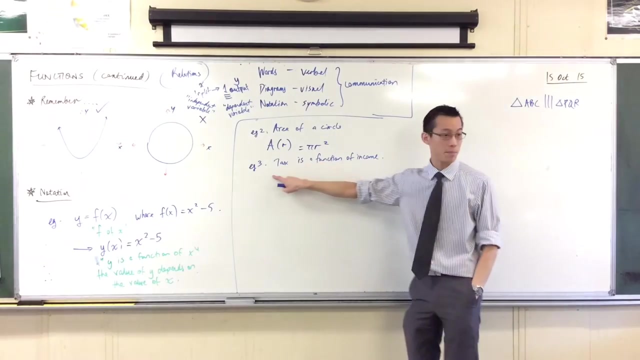 There we go. It's a little bit rarer. you can see what's going on, Can you see? you see that like enormous, awkward table that you've seen before up there, Taxable income, Tax on this income. It's long and it's complicated, That thing. that's a function. It's a messy function, right, But all it does is it takes two variables. It takes an input. you tell me how much money you earn and I'll give you an output. I'll tell you how much the government is scraping off you right, It's a simple connection between two variables, right? Independent and dependent. okay, Let me give you a couple of other ones that you're familiar with, just to extend this a little bit. 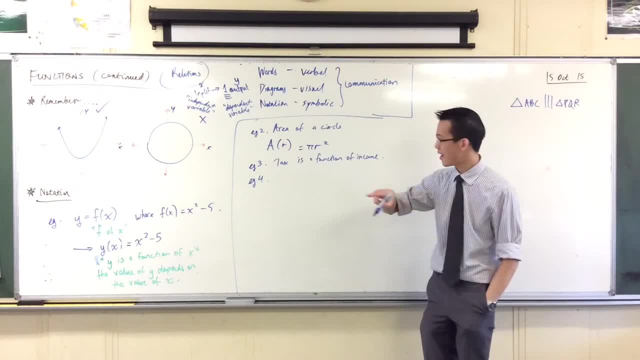 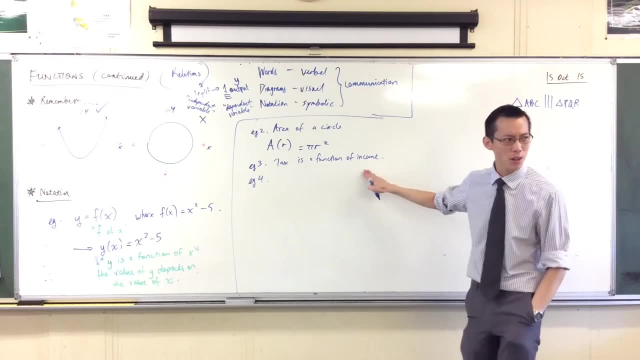 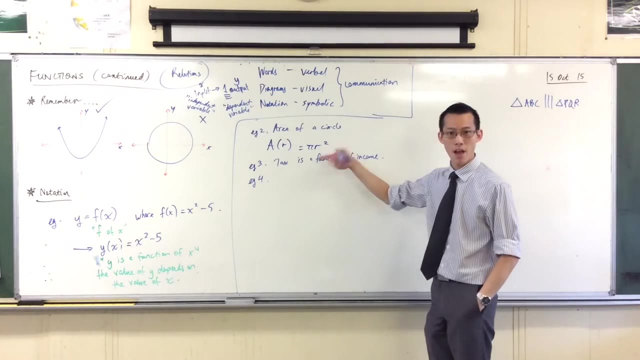 I've given you one, two, three examples where there is one dependent variable and one independent variable. But as you know lots of things in life and lots of things in mathematics, they don't just depend on one value at the end. One value at the end, right, For instance, area of a circle. How about the volume of a cylinder? Here's another example: right, What's the formula for the volume of a cylinder? 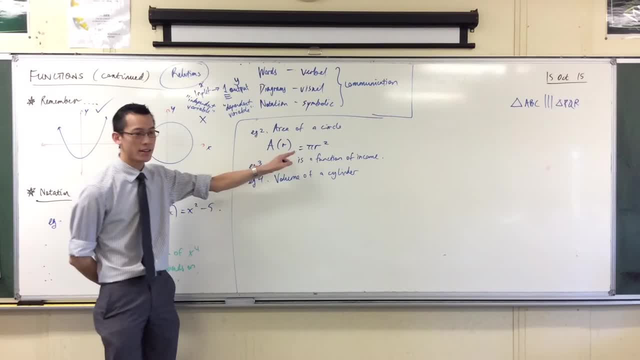 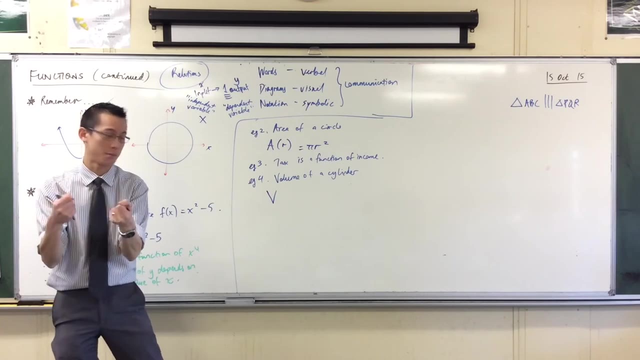 It's pi r squared h. I need the height of this thing right. So when I write v, volume is not just a function of radius, It's also a function of height, And it's not just one or the other, it's both at the same time. 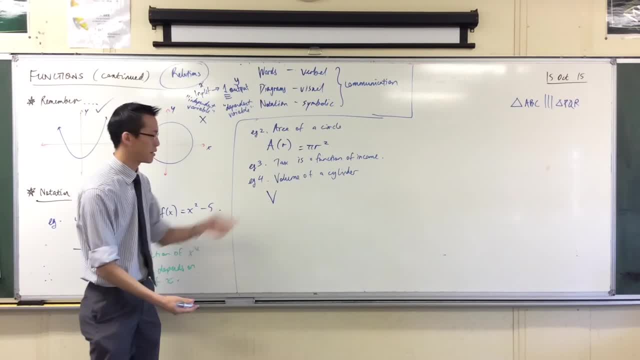 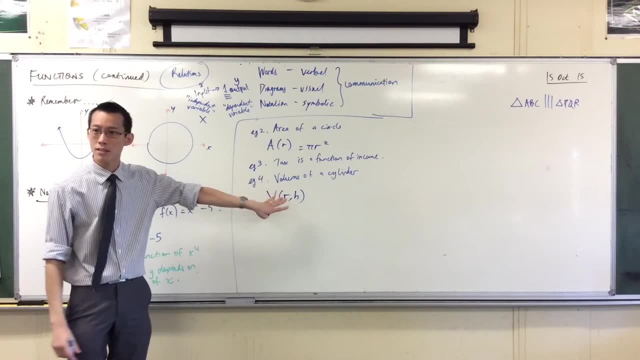 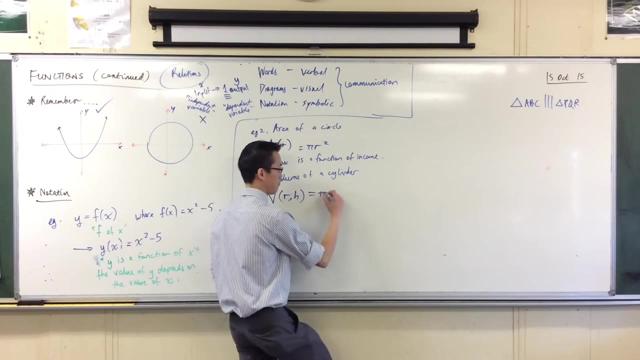 So not that you need to necessarily know this for the next test that's coming up, but it's a natural extension of this Volume is a function of r and h. That's all it means. right, You need to give me two numbers. right, You need to give me two inputs and then I'll tell you the output. And, of course, it's like you said: pi r squared h, right? 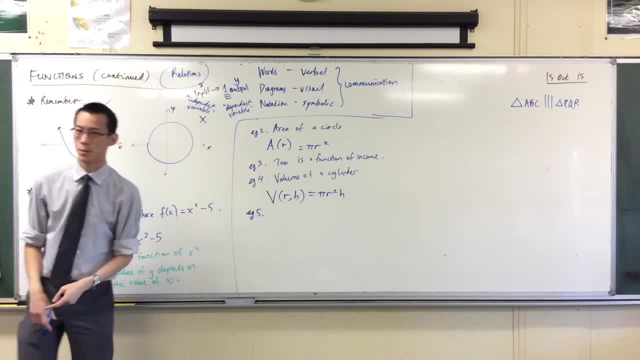 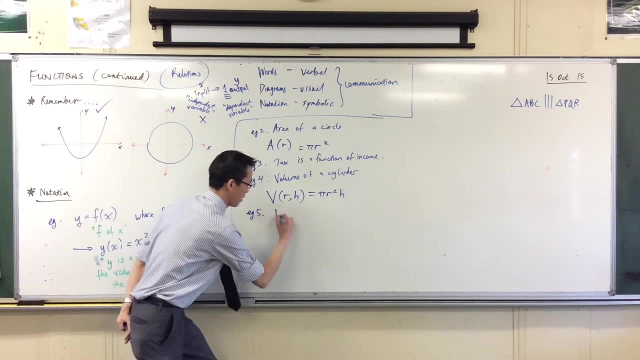 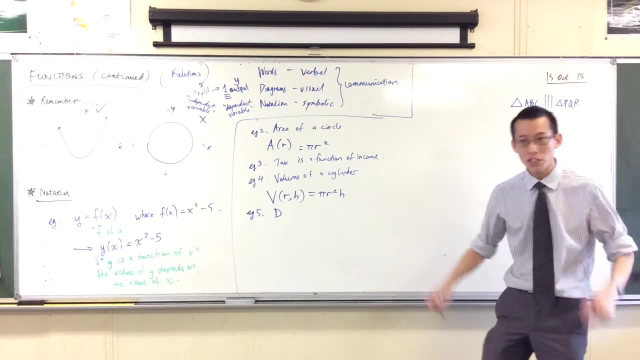 How about? I'm not even going to write the definition for this one. If I'm in a car, right, And I want to know how far have I traveled, What's the distance traveled? I'm saying distance, right. What is distance? Think in your science head, right Physics. What's distance? a function of? What two inputs am I going to put into that? I need speed and I need time right. 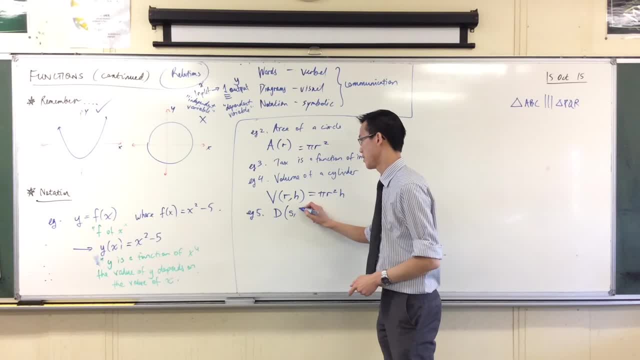 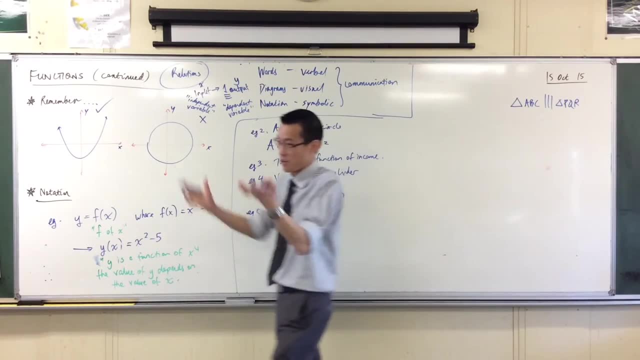 Right. So I would say distance is a function of speed and time, right? It's a very simple one, It's just speed times, time, right. 60 kilometers an hour, traveling for three hours, three times 60,, 180 kilometers is how far you've gone, okay. 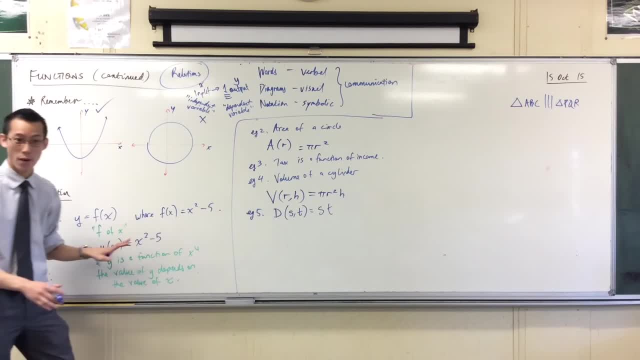 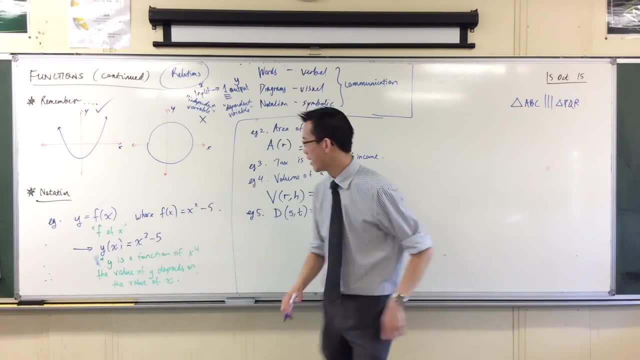 So this is a simple, simple idea, right? And this is how we're writing it. Now let me come back to my very, very first example, because x's and y's are where we're going to spend most of our time. okay, 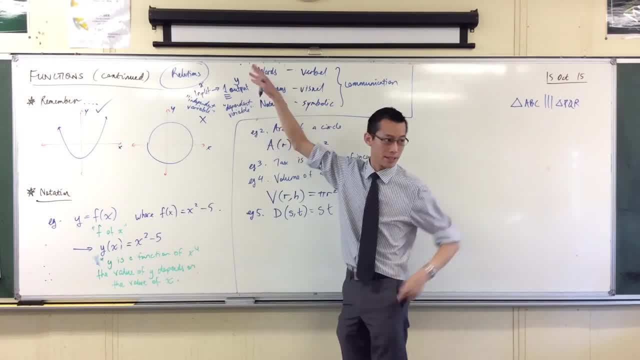 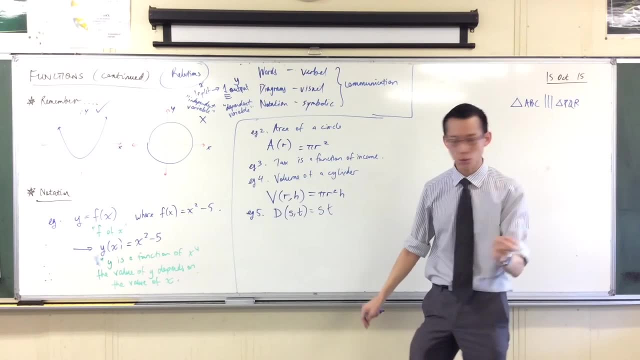 There's a natural way to think about this and actually not just think about, like all of these. There's a very, very abstract. who knows what these things are? equal to right, But I can think of these as a. I can think of this notation as a tool for use: subheading, substituting and evaluating. 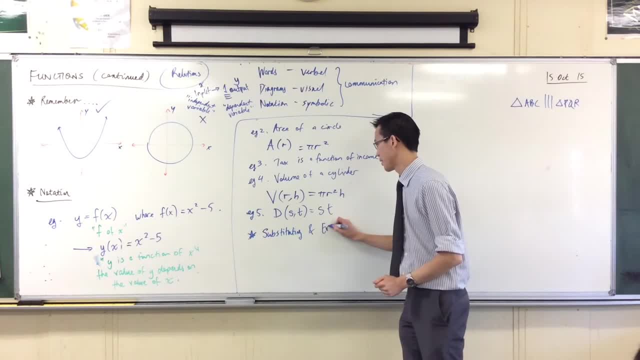 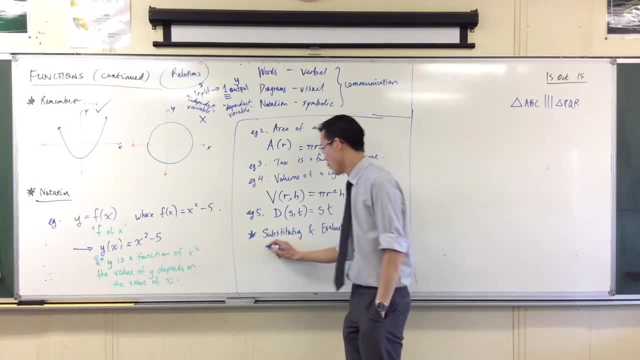 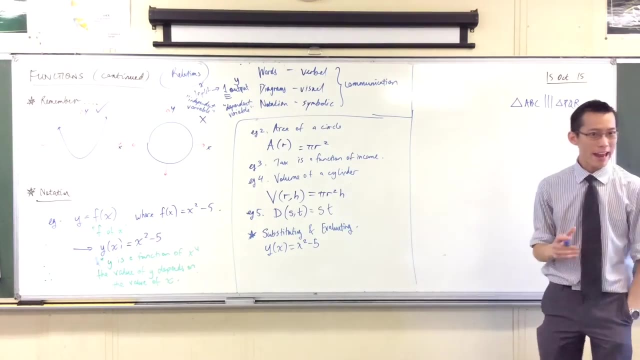 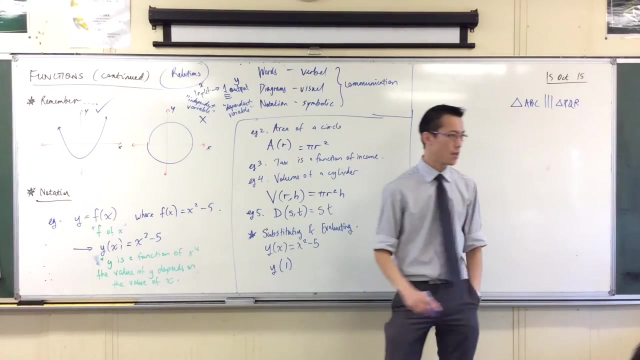 Substituting and evaluating. So if I come back to this guy right, y of x equals x squared minus 5, okay, Just human, Just human, right. If I wrote down this, the first line says y of x. is that What? would you read that as: 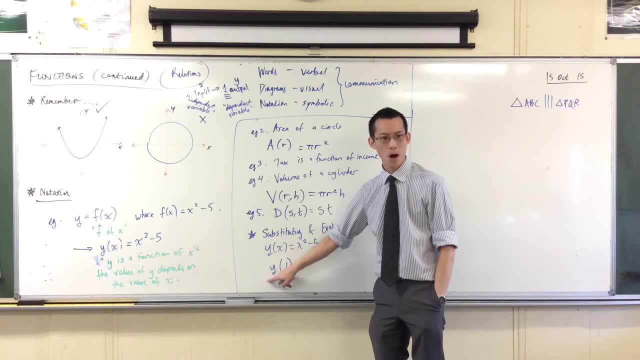 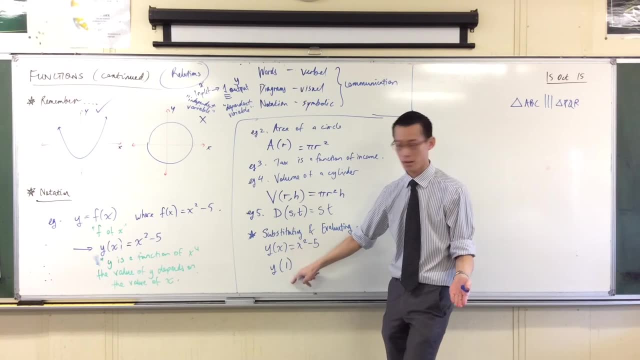 You wouldn't say y of x, you would say y of 1, right, y of 1.. And everywhere you see an x, you're just going to put a 1 instead. yeah, So this would be 1 squared. take away 5, which is just negative. 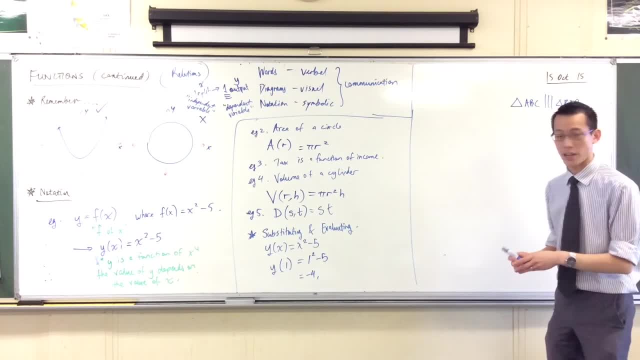 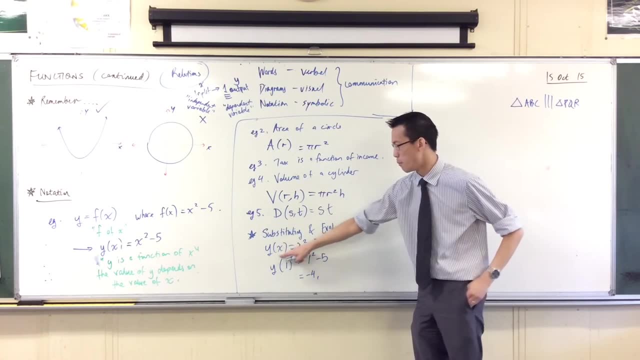 Okay, Now, what does this mean? What have I just done here? Two things: I've substituted in a value of x. I've swapped out, I've switched out all my x's for 1's. If I had like more x terms over here, like x squared minus 3x minus 5, all of those x's over there, I'd also put 1's in there. 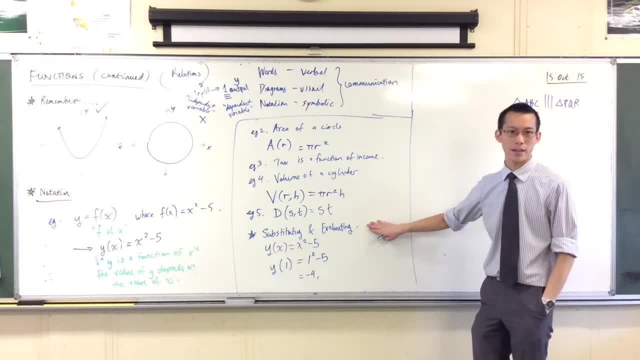 Okay, so I've substituted. And then, secondly, I've evaluated. okay, I've gone and crunched the numbers and that's what I've got, Okay. So another way of reading that we say: okay, I've substituted. 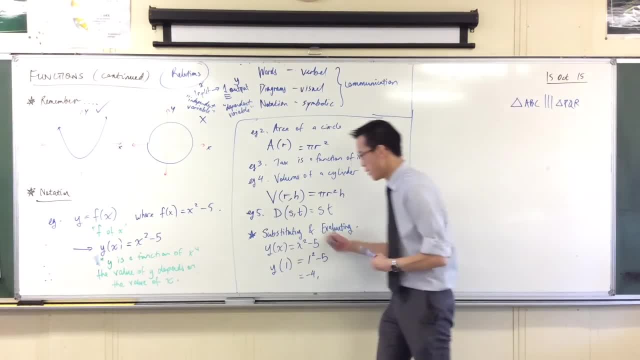 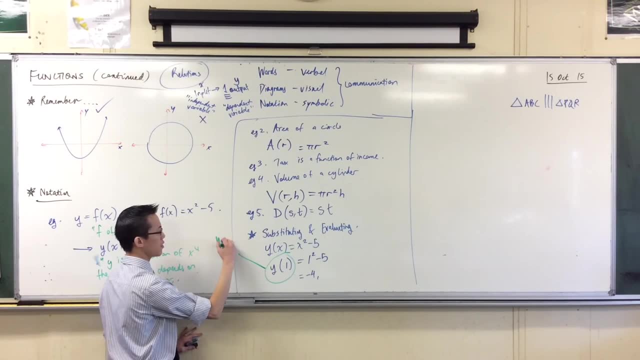 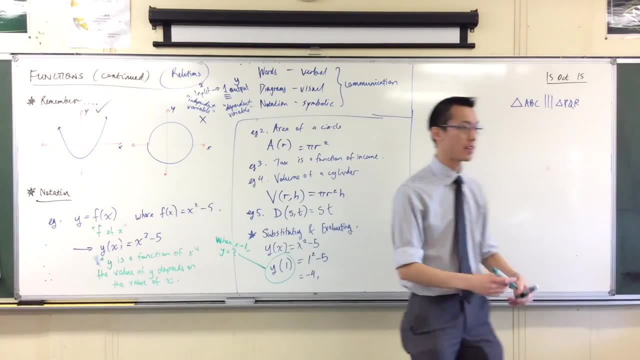 Another way of reading that we said y of 1, that's correct. But another way of reading that is, when x is 1, what's y equal to? Okay, When x equals 1, y equals what. That's what this question is answering, right. 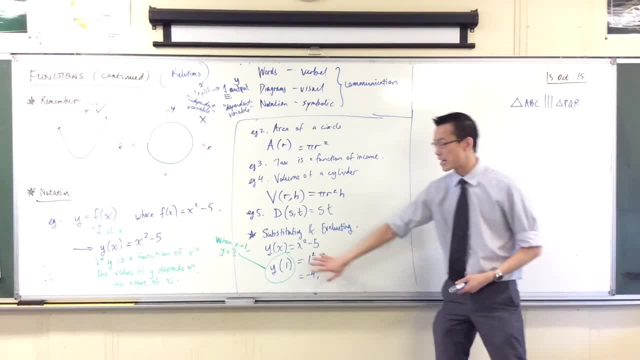 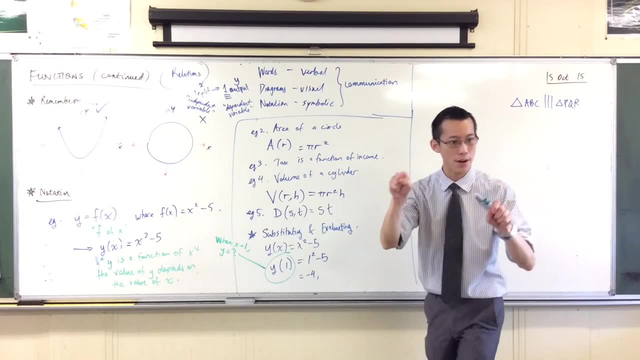 This answer is a question. whatever it is okay. That's what you're interested in And, correspondingly, this is giving you coordinates. Do you see? this is giving you coordinates. It's giving you a pair of numbers. What's the x that I've got? 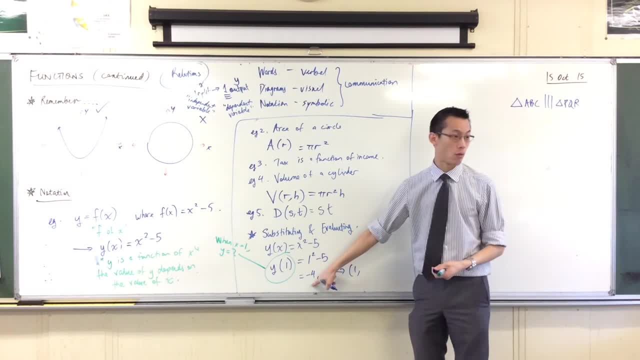 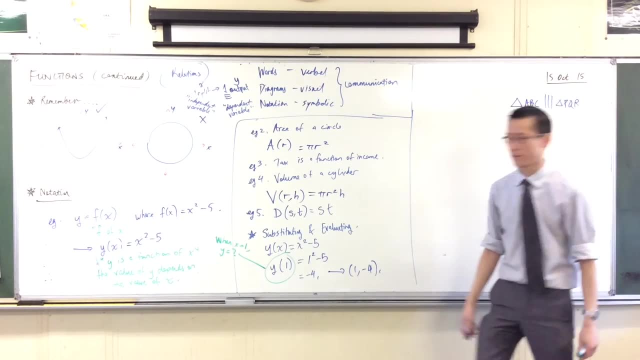 It's just 1, right And the corresponding y value right, The output I'm getting is negative 4.. So 1, negative 4 is a point on my curve right? I guess it'd be, I don't know there. 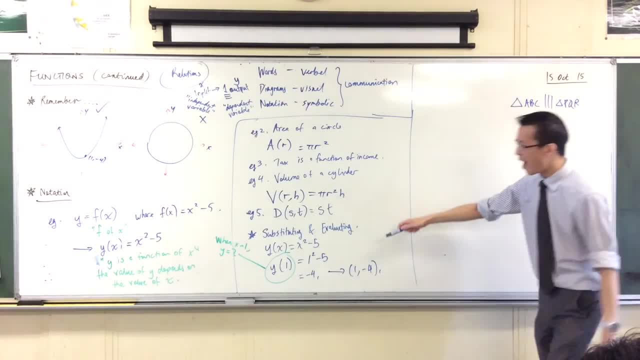 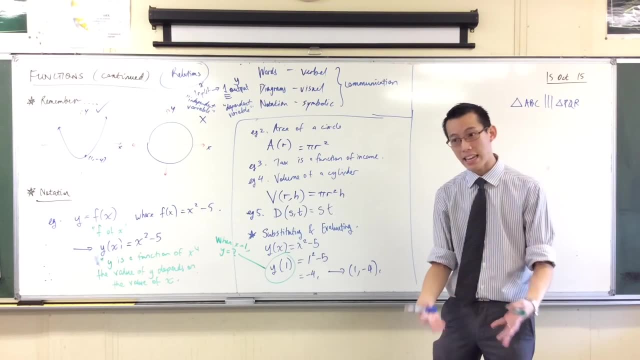 There you go. So all I'm doing is popping in numbers. Now I can do this for anything I like. I can do it for y of 1,. I can do it for y of 100.. I can even do it for more algebra. 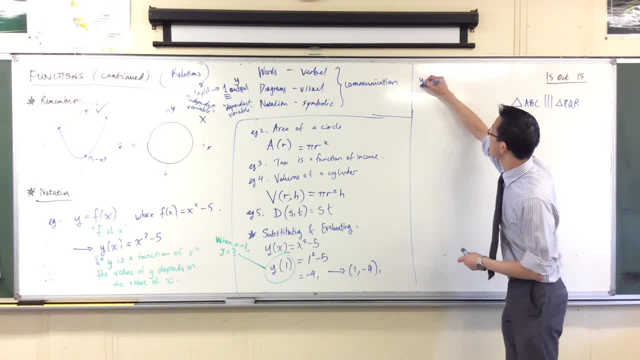 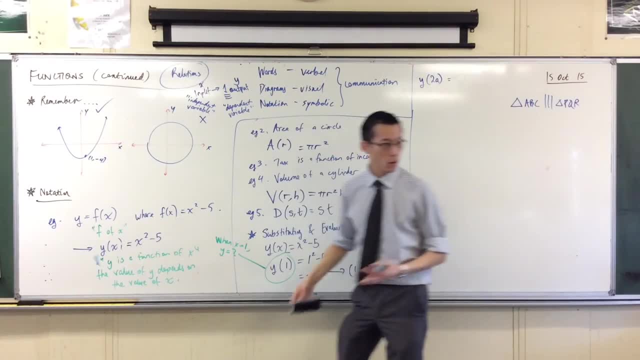 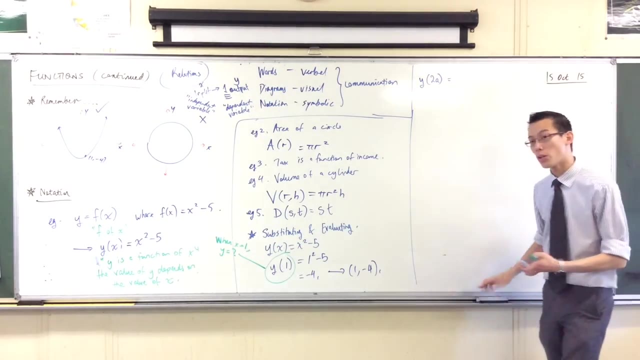 If that's useful to you. For instance, if I say what's this equal to y of 2a? Well, it's asking: when x is equal to 2a, What's y equal to? okay? So all I need to do is just like I did before: straight substitution, right. 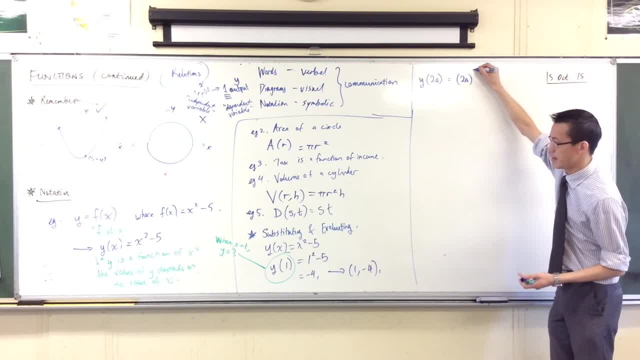 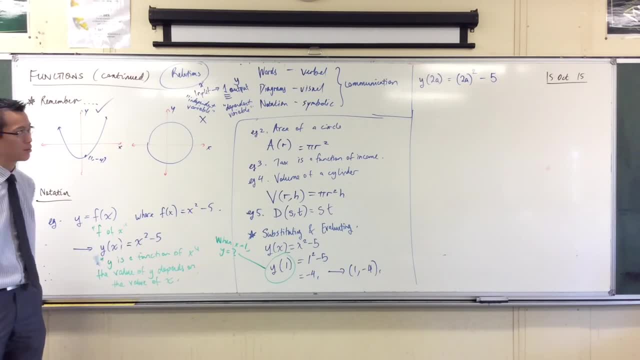 Let's see here: I've got 2a in there squared. take away 5, right. Note the brackets. okay, They're really important Because the whole thing is getting squared right. What is 2a squared? 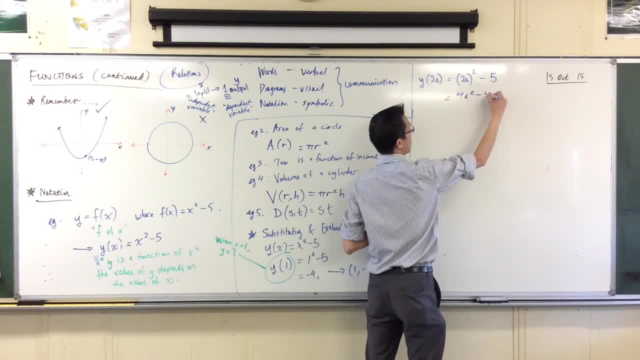 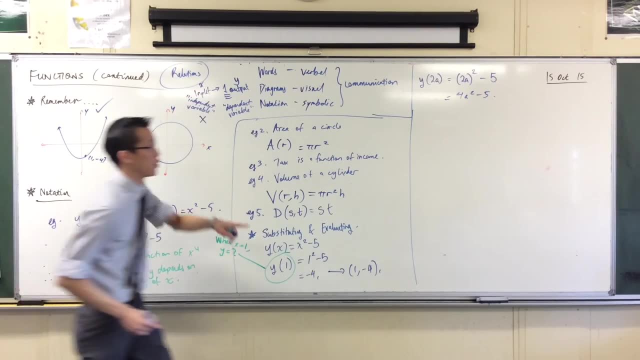 4a squared right. So I don't know what that value is, but that's because I don't know what a is. But if I did, I would just pop that in Now. I know that 2a- 4a squared minus 5,. 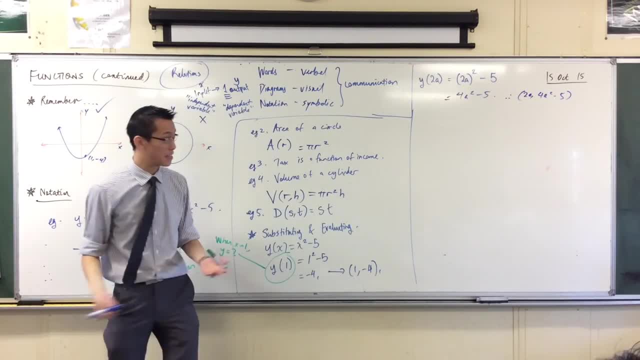 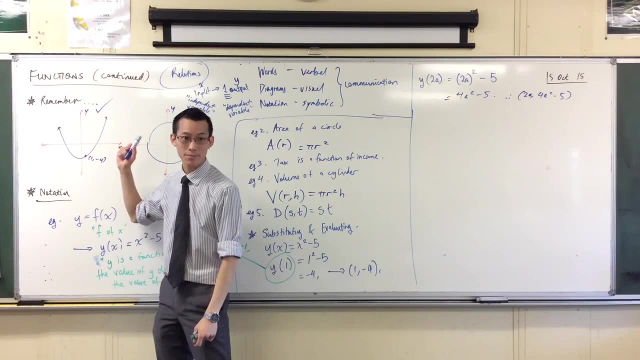 that's also a point that's on my parabola. I have no idea where it is because I don't know what a is, But that point for any value of a is going to be a point on my parabola, right.